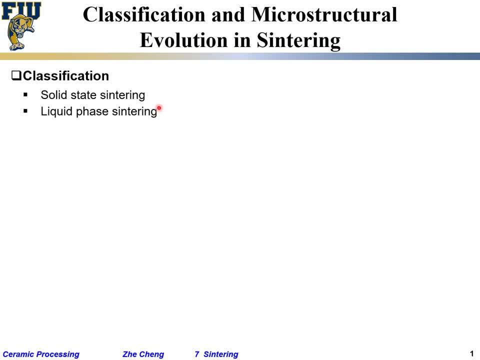 Liquid-phase. SYNTRIN is still. the majority of your material is still solid. but there are liquid phase that helps the mass transport process, help lowering the sintering temperature. okay, so both are common. okay. liquid phase sintering occurs for those systems that are difficult to. 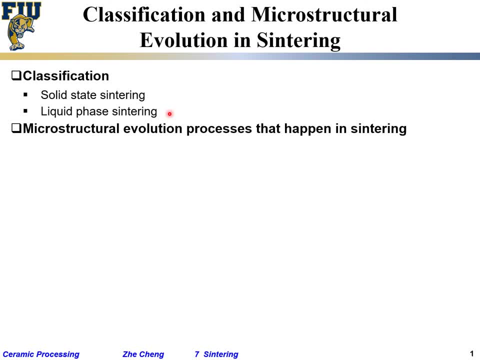 sinter by solid state sintering. okay, microstructure evolution. that can happen in sintering. the first one people call densification, which i show something like this: before the sintering happens, we have individual, separated particles and after sintering the particles probably change shape, but they they come together. that's not much porosity. 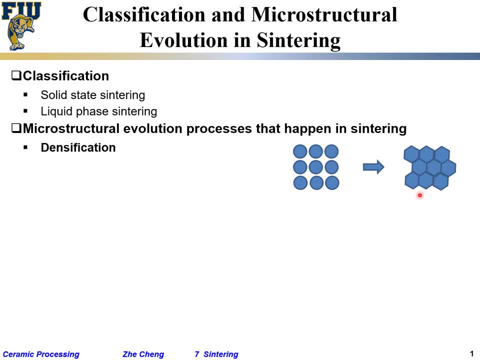 that's the ideal situation. ideal situation, okay. remember we said: three green colors together, okay, 120 degree, okay. and then the bonding particles, with elimination of pores. we want to get rid of the inter-particle porosity. another type of structural evolution that quite often occur at the same time is called green growth. okay, which is i have, let's say. 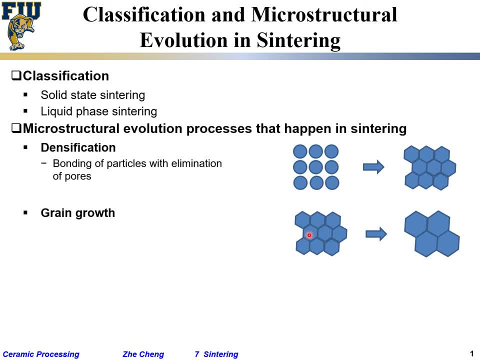 sintered or completely sintered particles, green size, certain size, certain dimension. if you hold for a little bit longer, the greens become larger. that's people call green girls, which is very, very common, especially if you achieve near full densification or full densification beyond. 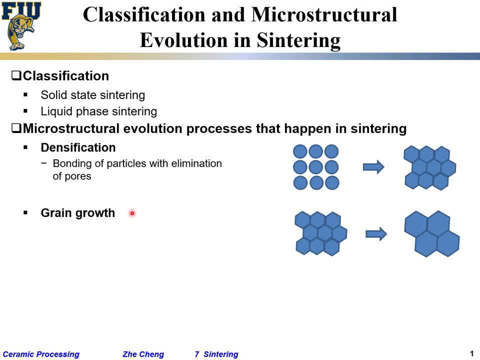 that the particles will grow a lot until it reaches very, very large. okay, bonded particles grow in size. a third one people call coccine, which is initially. we have individual, separated small particles. after heat treatment i have pretty much separated large particles but i have not really eliminated for all between them.